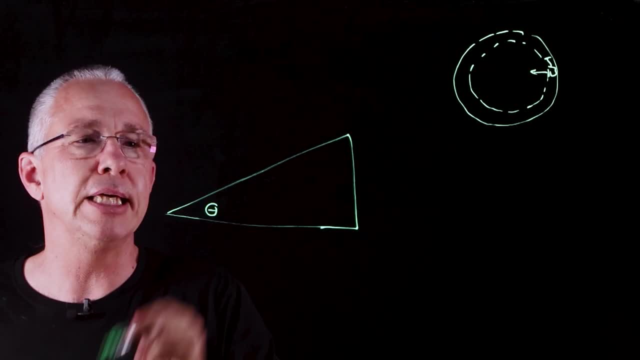 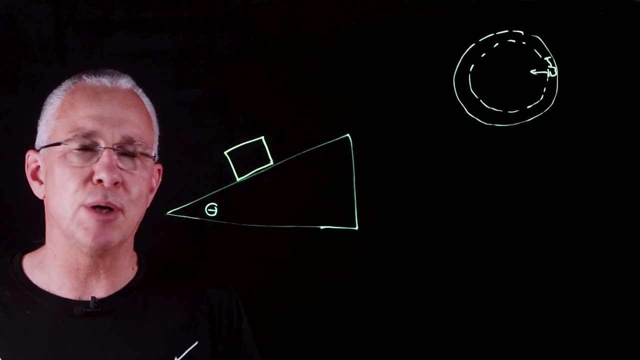 the angle, in this case, of our banked curve, and that's going to be the angle that we have here. We'll need our car over here, and I'm just going to do what all physicists do: simplify things by drawing rectangles. And then we ask ourselves the question: what are the forces? 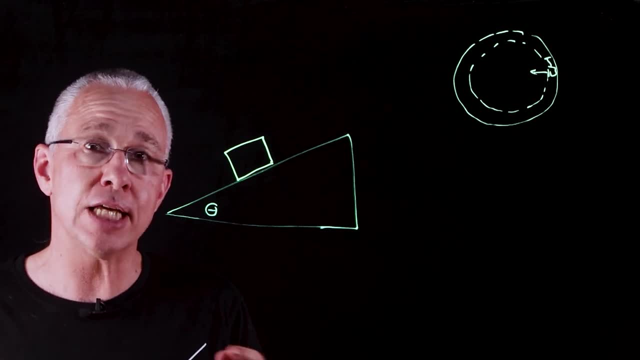 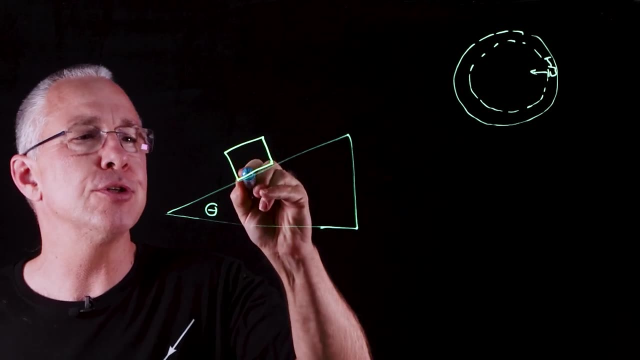 acting on the particular car And in our case, we're going to simplify it by ignoring frictional forces. at this stage, We're going to keep it nice and simple And we have two basic forces. The first is, of course, the force due to its weight, or mg. 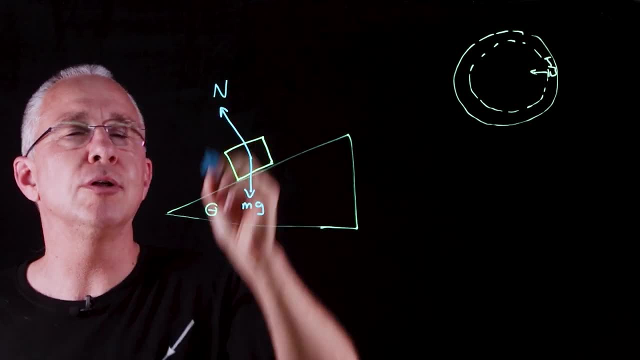 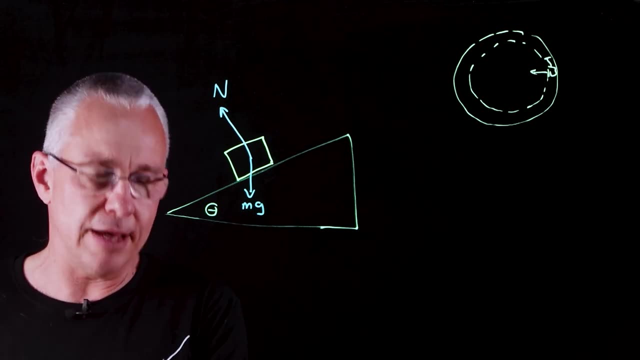 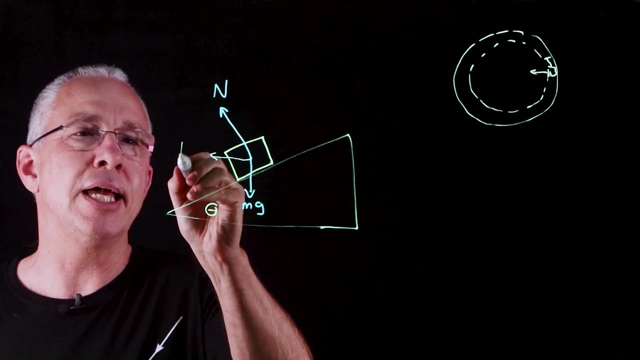 And the second force is the force, that is the normal force acting in that direction. Now you can see now that those two forces, if they add up, we get a value that is the sum total of those forces which is going to be a direction in that point there, And that ends up being the 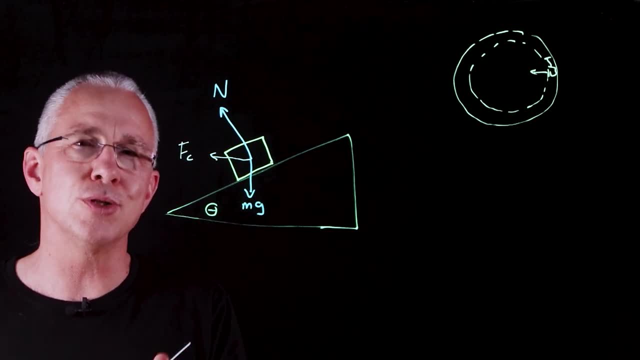 centripetal force. So, in other words, the centripetal force is the result of those two forces acting. Again, remember, we're not including friction in this particular analogy. So we're just going to use the force that's acting on the car and then we're going to 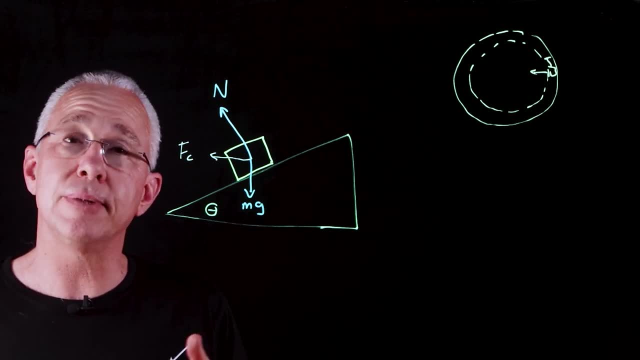 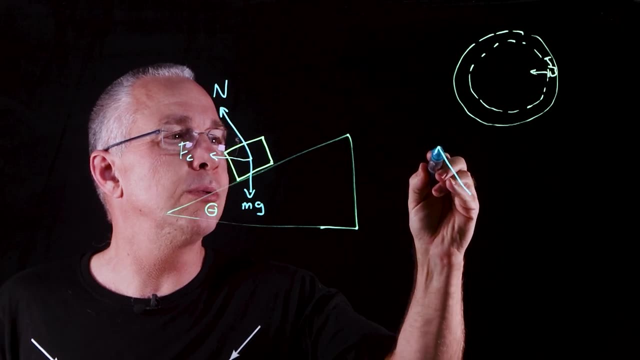 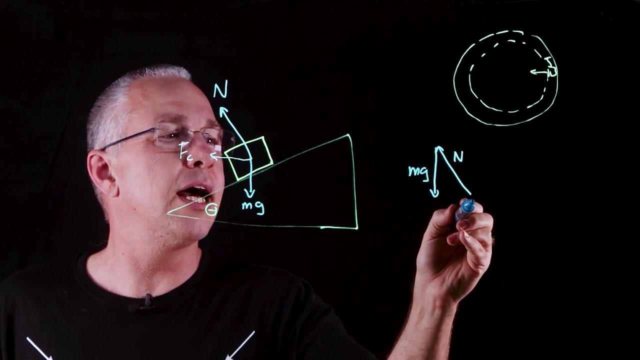 simplify the process. Now, how do we therefore combine those things? And there's a couple of ways that we can do this, And one of them is simply by drawing a nice vector diagram. And so, for example, if I have my vector of my normal in this direction, I have my vector of my 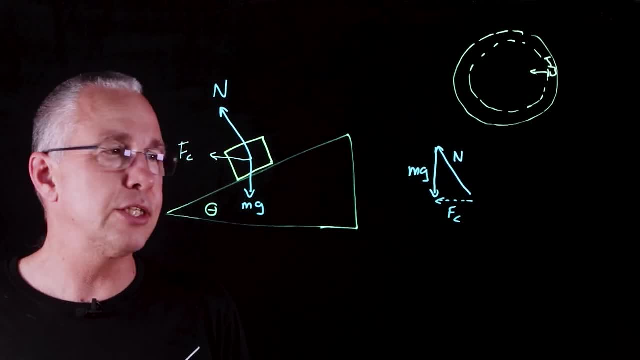 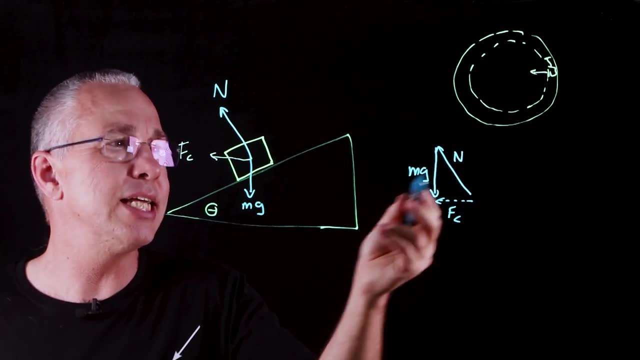 mg in that direction. I then have my net force, which is fc in that direction, like so, And what I'm going to do is I'm going to add that vector to my normal and I'm going to give that vector a name, So that's going to be a function of fc in that direction. Now what we can do is we can. 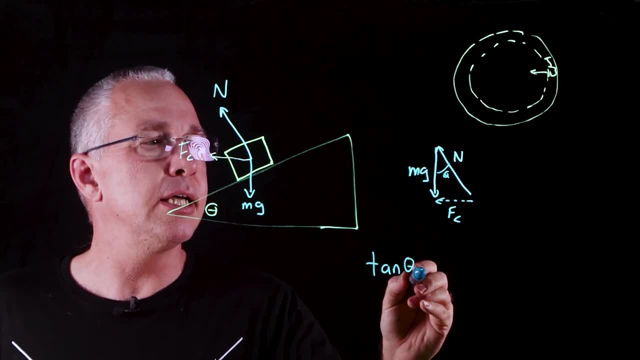 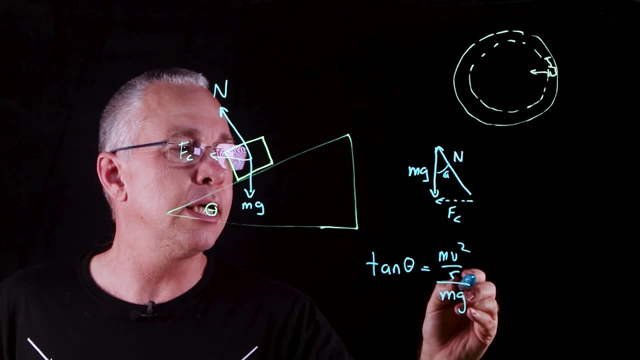 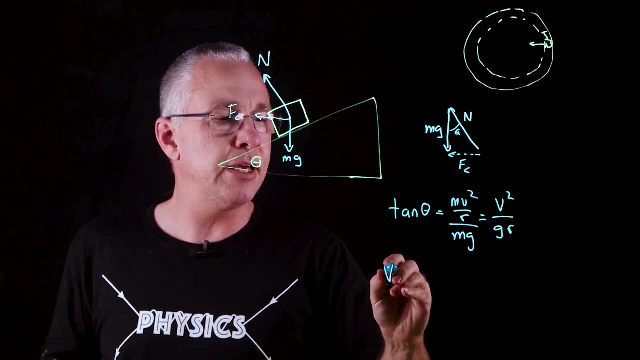 write that down here in a little bit. We can write out mathematically the relationship with this, And that is because this angle right here happens to be this angle right there, And so now what we can see is that we have the tan of theta is equal to the centripetal force, which is m v squared over. 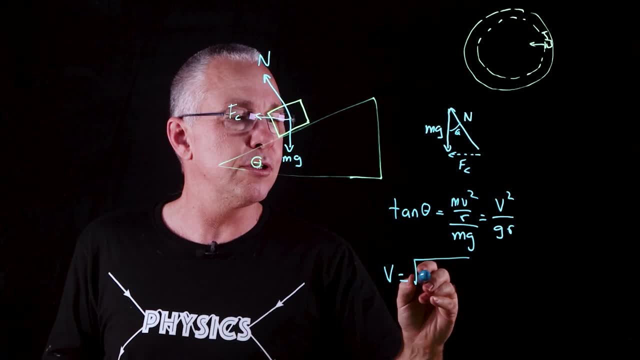 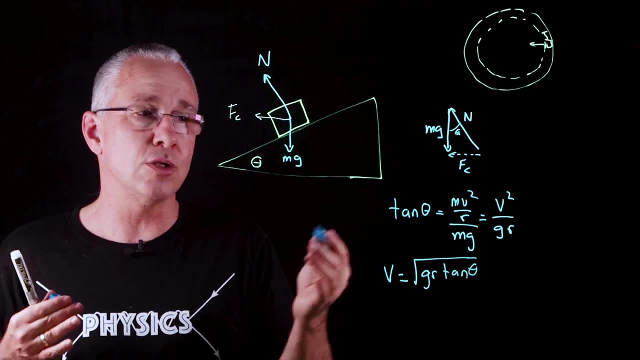 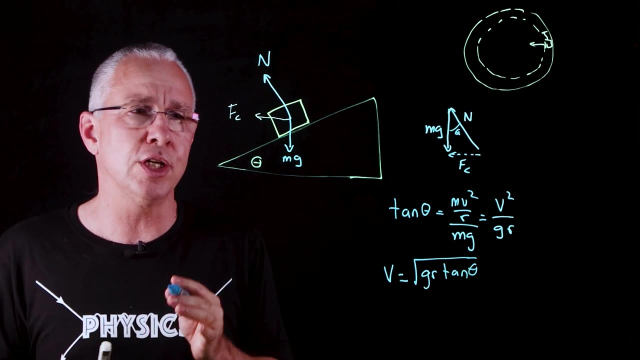 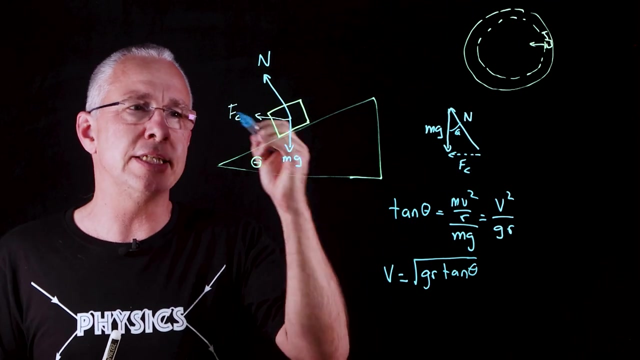 r divided by mg, g, r tan theta. what you notice straight away is that the mass is not in the formula anymore. what we say is: it is independent of mass. the velocity of an object that is able to stay in circular motion is not dependent on its mass itself. in this particular case, if the velocity increases, 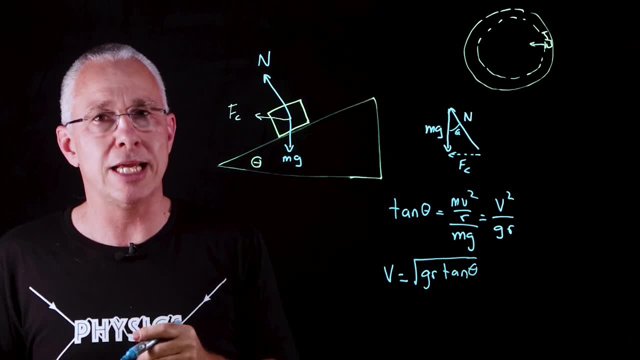 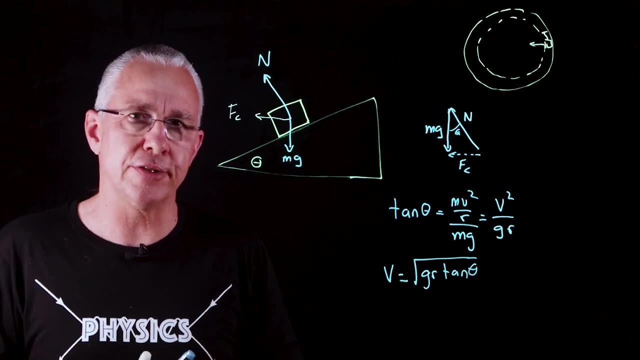 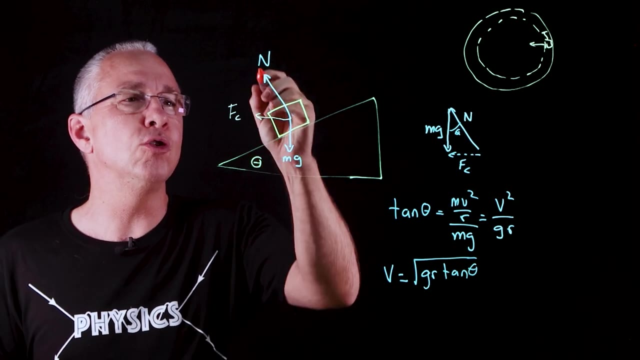 it will slide up the hill. if the velocity decreases, it will slide down the hill, but mass plays no part. now, that's one way of trying to resolve it and we use victor analysis. but i want to quickly touch base also on a component way of doing this. you can see that the normal has two. 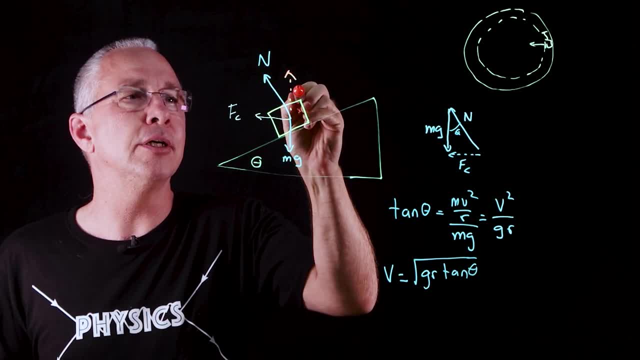 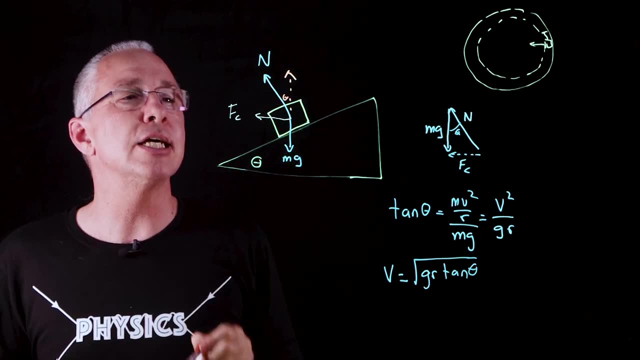 components. it has a vertical component. in this case, if this is angle right, here is the value theta, then this becomes theta as well, and then, of course, we have our horizontal component, which is this component there, and you can see, you can see that the value of theta is the value of theta and you can see that the value of theta. 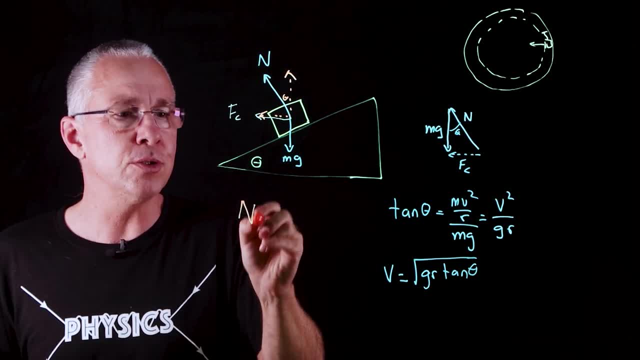 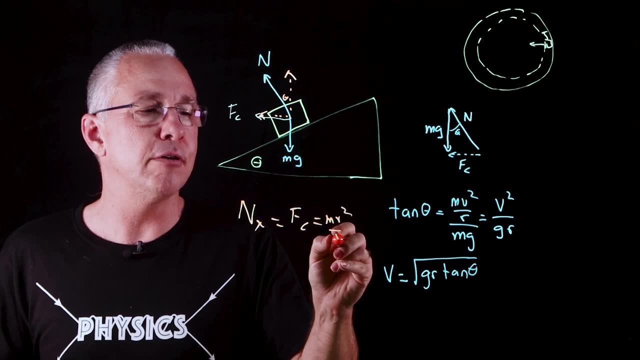 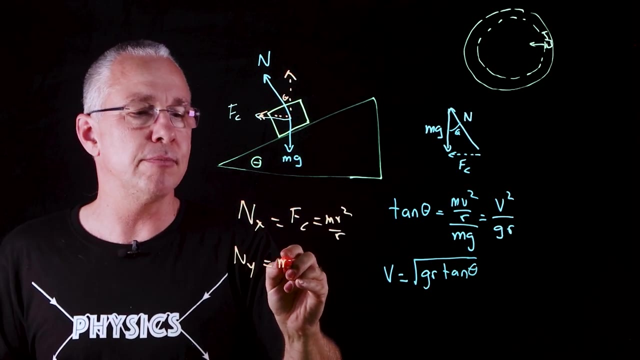 is straight away that the normal's horizontal component- let's call this nx- happens to be the centripetal force, which we know is mv squared over r. what about the vertical? well, you can see, in that case my vertical component is equal to mg, because we have a net force, in this case, of zero. now, nx. 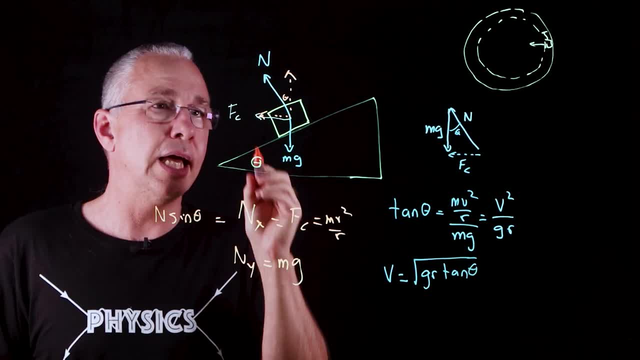 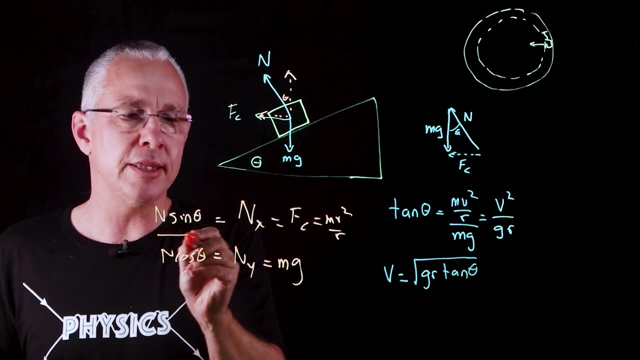 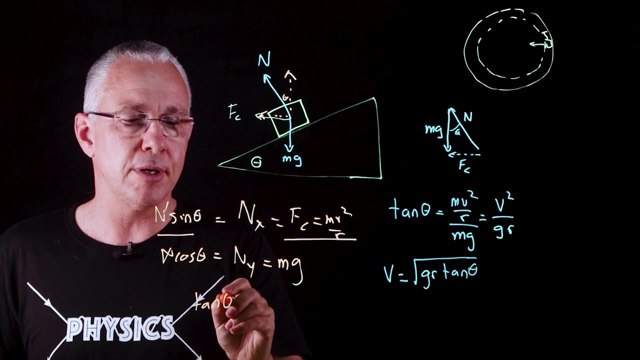 ends up being n? sine theta and ny ends up being n? cosine theta. and now what you can see is: well, if i divide this and then divide this, you'll see my ends cancel out. i have tan theta on the bottom over here and then over here, i end up getting exactly the same i had. 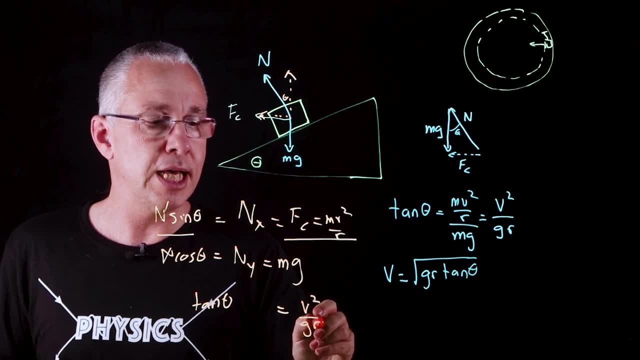 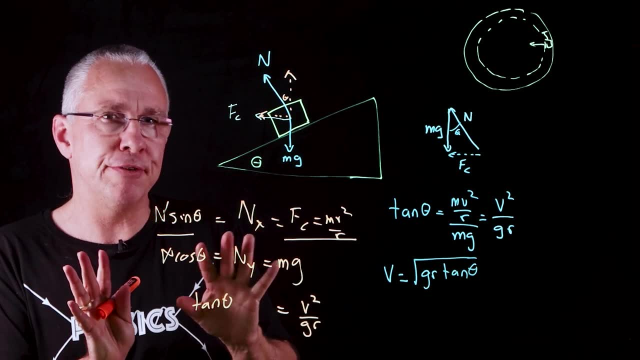 before, and that is v squared over gr, and i get exactly the same relationship i had before, but this time we did component analysis. now, if i were to add friction to this, this becomes a little bit more complex, and generally in high school you don't necessarily know how to do this. so i'm going to 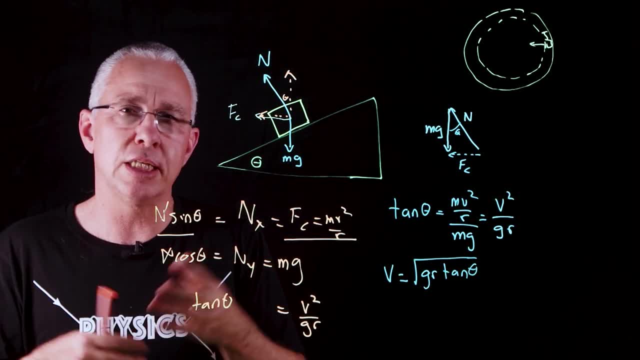 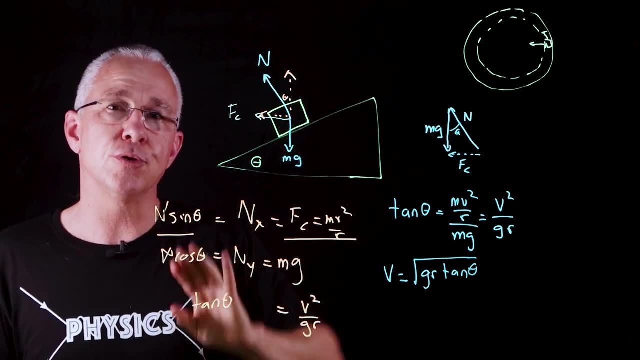 need to be able to do that in exam conditions because it's a little bit more involved, but the principles is exactly the same. you would just simply add a vector of the frictional force direction. in this case, it is either going up the plane or down the plane automatically. you actually